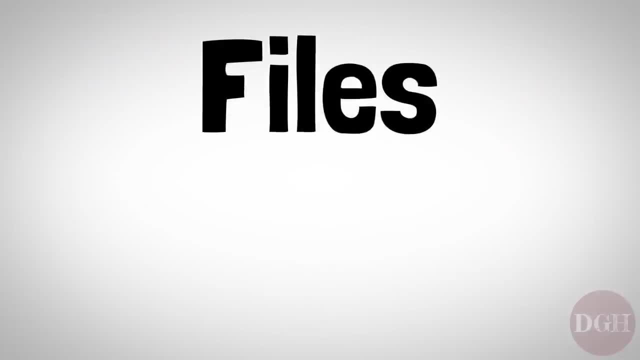 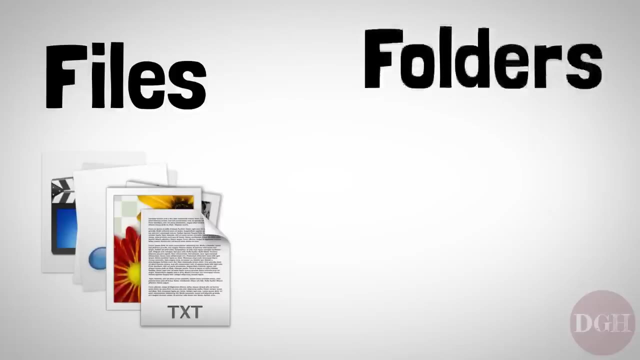 stored as files. A file is basically a chunk of a certain kind of data. There are many kinds of files, including video files, audio files, image files, text files and many, many more. In order to keep files organized, we use folders- A folder on your computer. 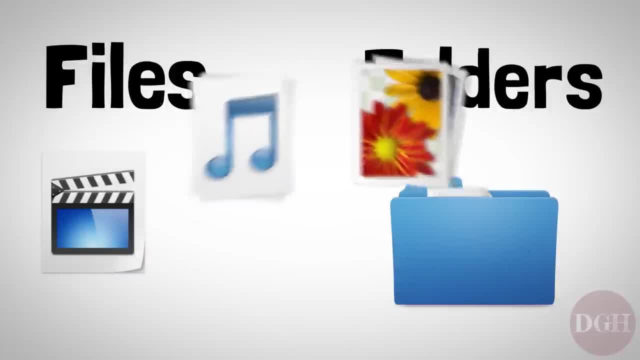 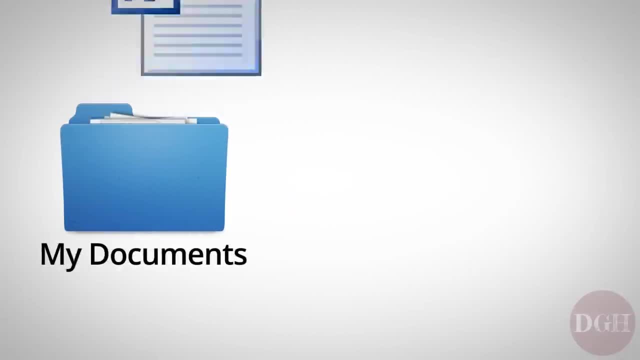 is just like a real life folder. It's a place you can put files, to separate them into groups that make sense. Every folder has a folder name And every file has a file name. The file name serves a couple purposes. The first purpose. 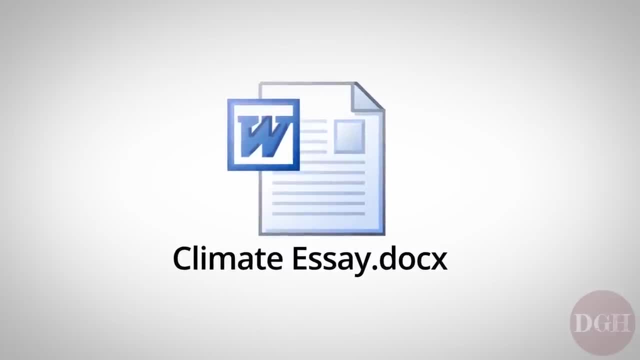 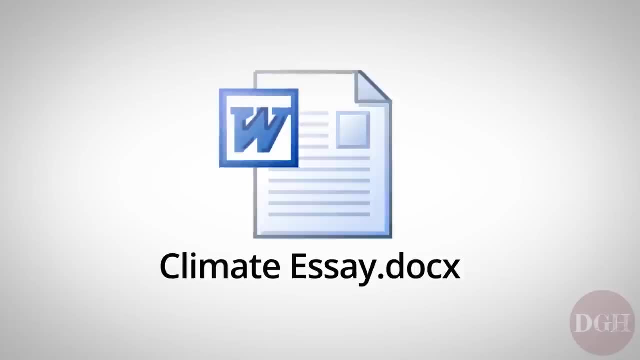 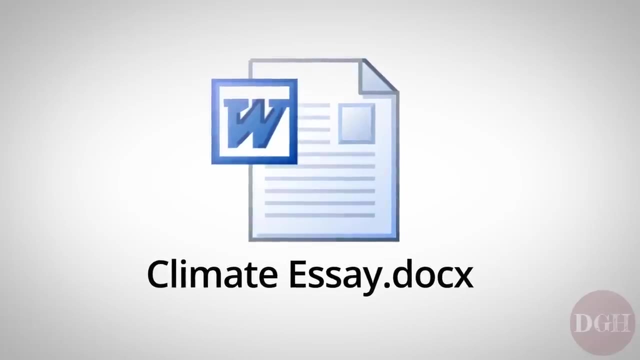 is to help you, the user, identify what that file is about. So if you wrote an essay about climate change, for example, you might name that file Climate Essay. The second purpose of the file name is to help the computer recognize what kind of file it is, so that it knows. 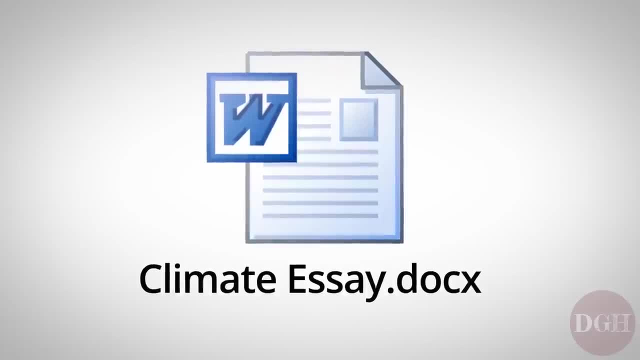 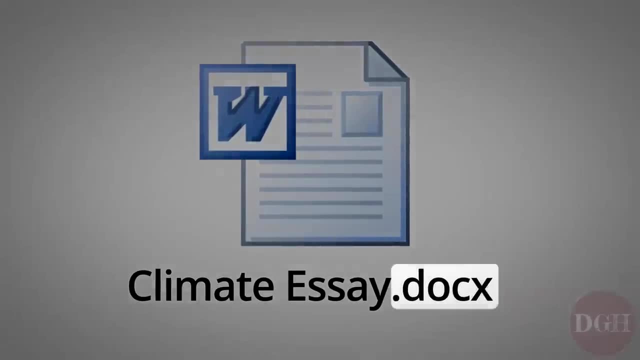 what program it should use to open it. There's a special part of the file name that is used for this purpose. It's called the file extension. At the end of every file name there's a period and then letters or numbers that come after it. Those letters or numbers are the file. 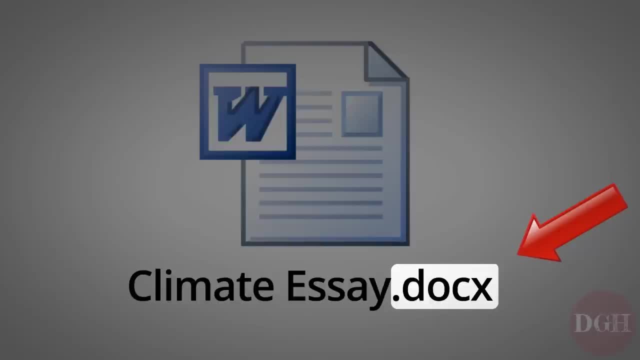 extension. The file extension is very important because without it, the computer doesn't know what kind of file it is or what to do with it. It's good to keep this in mind when you rename a file, because if you accidentally change or remove the file extension, your 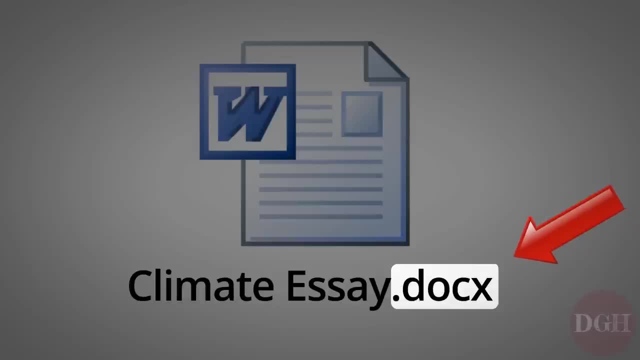 computer will not be able to recognize what kind of file it is. The file extension is a very important part of the file name. The computer might not be able to open it anymore and you'll have to rename it again and put the file extension back in order to fix the. 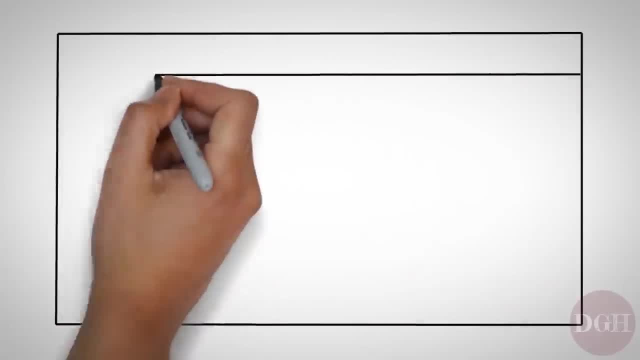 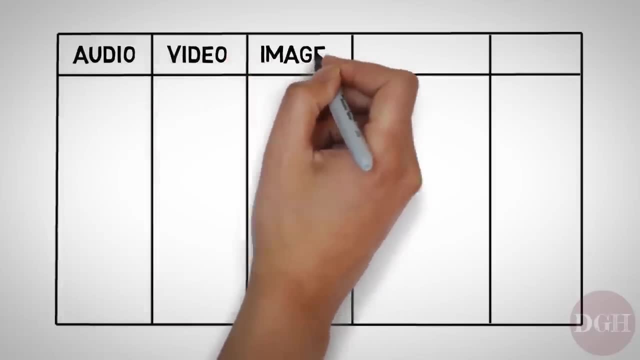 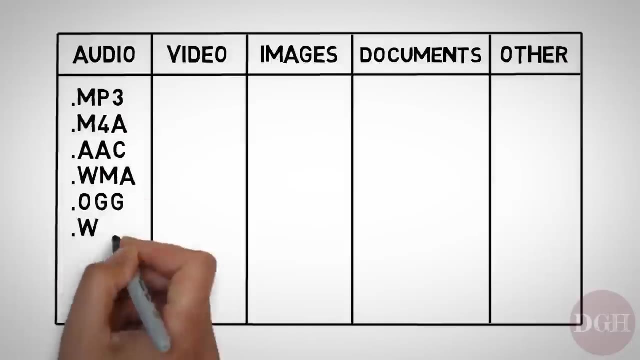 problem. Let's look at some common file extensions, grouped by category. We've got some that are for audio, some are for video, some that are for images, some that are for a variety of types of documents and then a few other important ones. This may look like a lot, but in reality 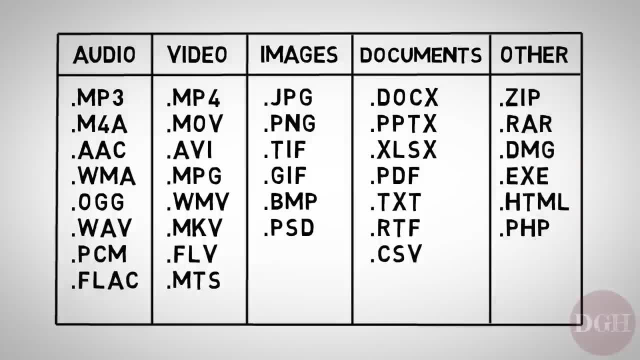 there are actually many, many more. You may be wondering why there are so many file extensions. Why are there a dozen different formats just to store one kind of data? The answer is that, even though they may store the same kind of data, they do it differently. For example, among the audio formats, some